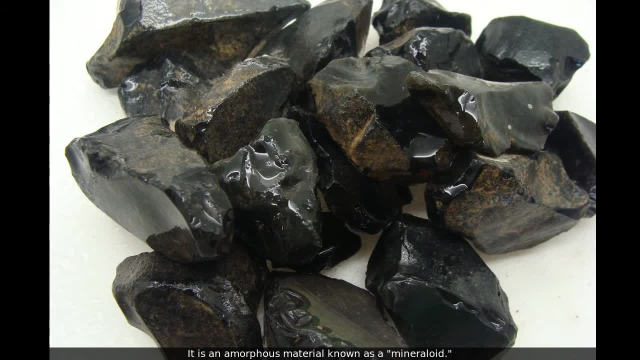 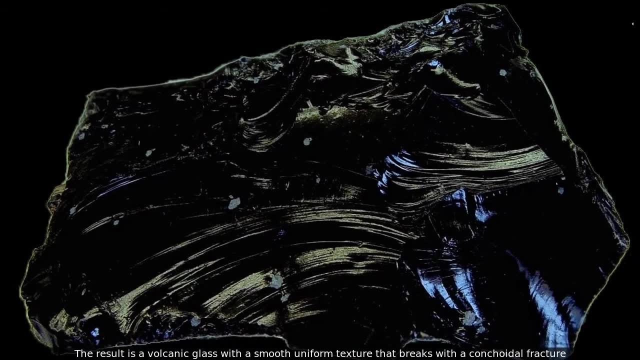 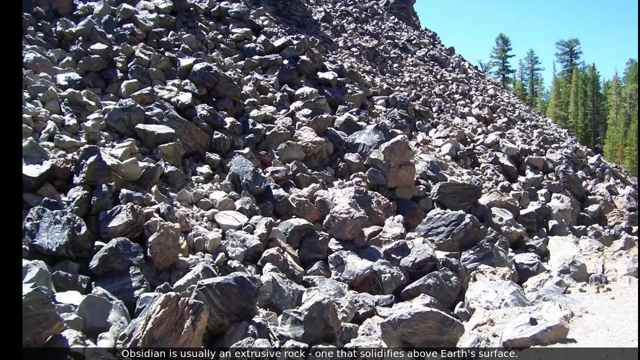 It is an amorphous material known as a mineraloid. The result is a volcanic glass with a smooth, uniform texture that breaks with a conchoidal fracture. Obsidian is usually an extrusive rock, one that solidifies above Earth's surface. 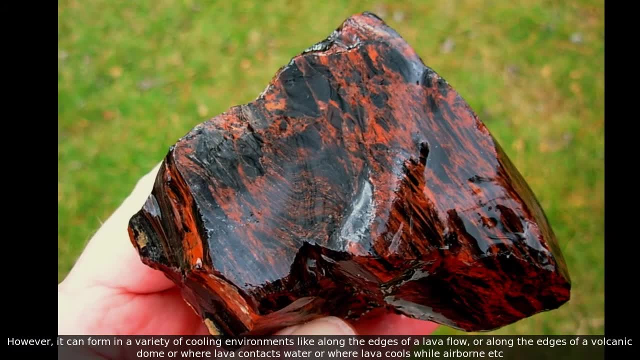 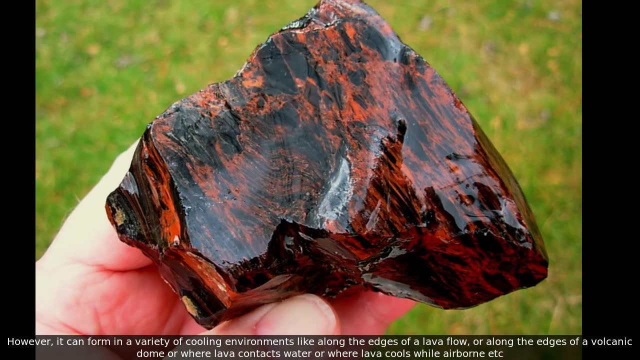 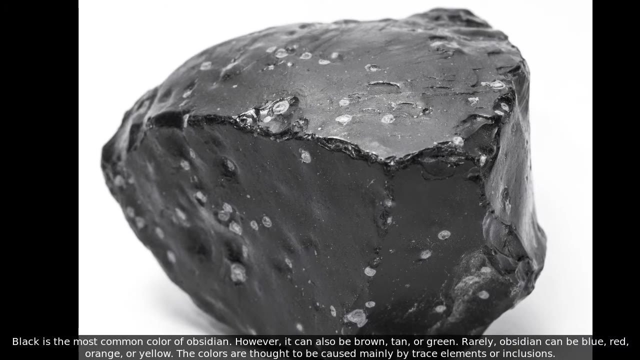 However, it can form in a variety of cooling environments, like along the edges of a lava flow or along the edges of a lava stream. It can also form a volcanic dome, or where lava contacts water, or where lava cools while airborne, etc. Black is the most common color of obsidian. 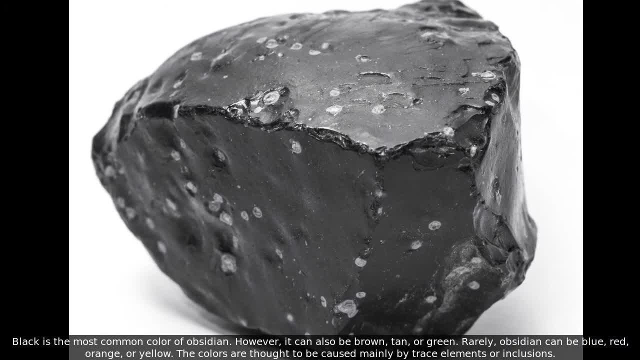 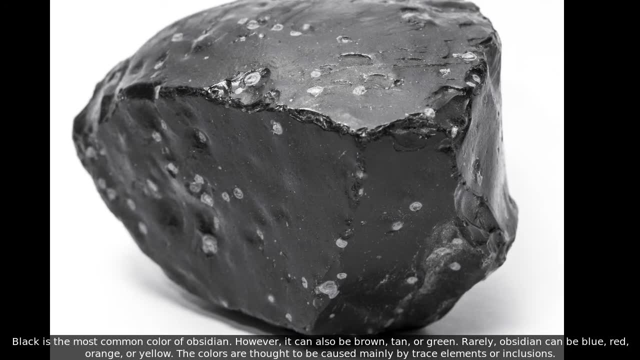 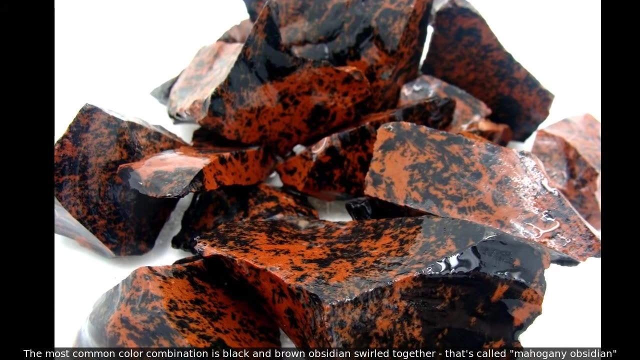 However, it can also be brown, tan or green. Rarely obsidian can be blue, red, orange or yellow. The colors are thought to be caused mainly by trace elements or inclusions. The most common color combination is black and brown obsidian swirled together. 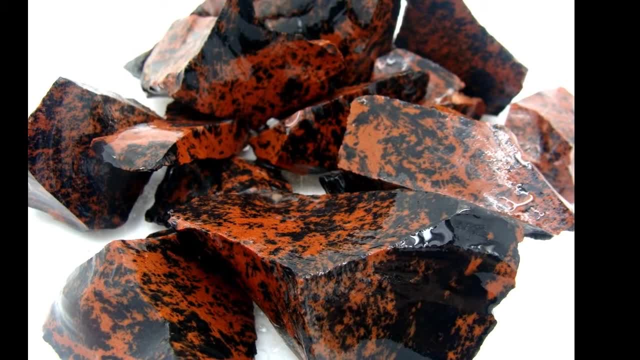 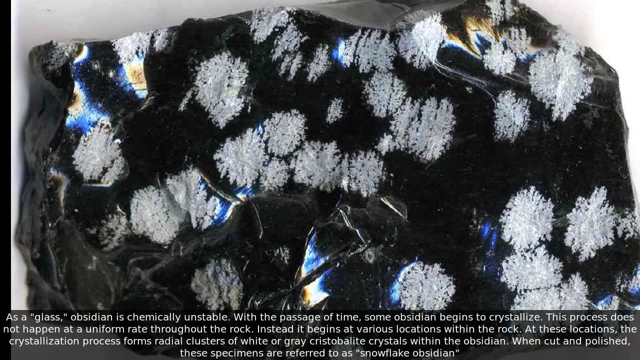 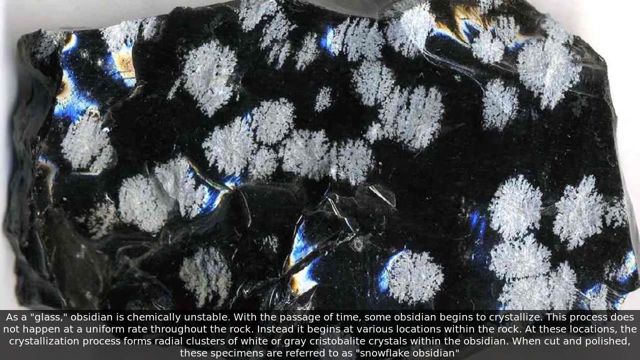 That's called mahogany obsidian, As a glass obsidian is chemically unstable. With the passage of time, some obsidian begins to crystallize. This process does not happen at a uniform rate throughout the rock. Instead, it begins at various locations within the rock. 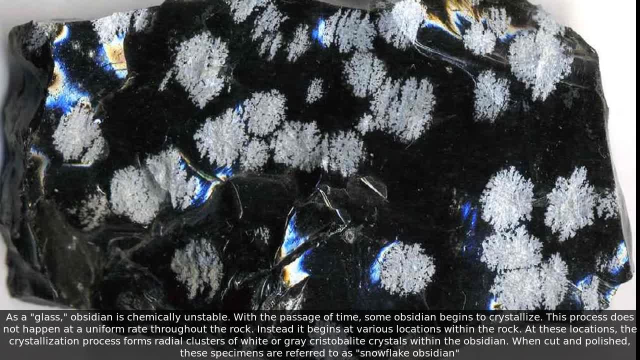 At these locations, the crystallization process forms radial clusters of white or gray cristobalite crystals within the obsidian. When cut and polished, these specimens are referred to as snowflakes. The black and gray cristobalite crystals form a radial cluster of white or gray cristobalite crystals within the obsidian. 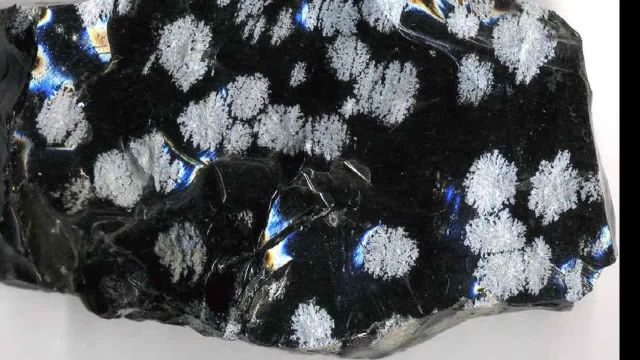 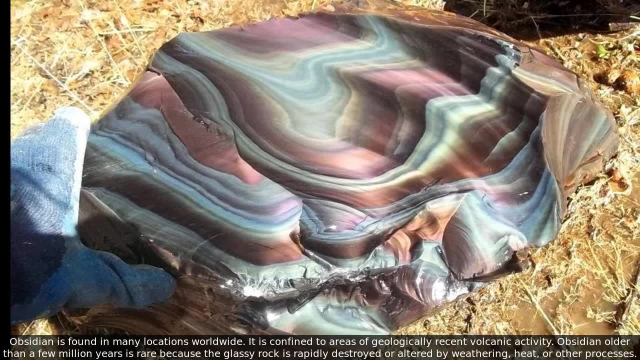 When cut and polished, these specimens are referred to as snowflakes. When cut and polished, these specimens are referred to as snowflakes. Obsidian is found in many locations worldwide. Obsidian is found in many locations worldwide. It is confined to areas of geologically recent volcanic activity. 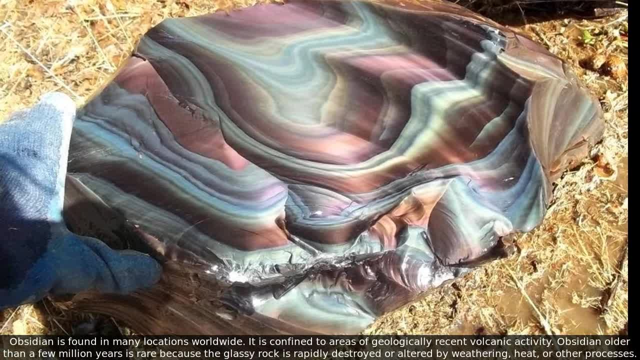 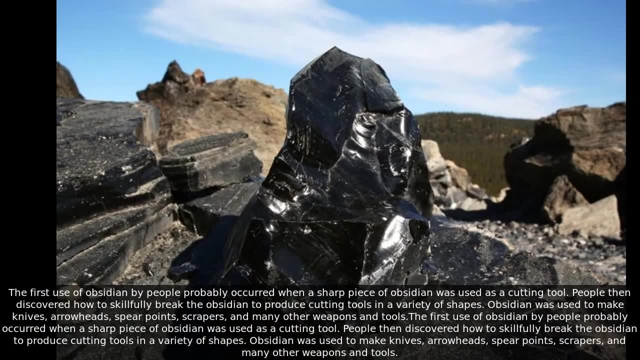 Obsidian older than a few million years is rare because the glassy rock is rapidly destroyed or altered by weathering, heat or other processes. The first use of obsidian by people probably occurred when a sharp piece of obsidian was used as a cutting tool. 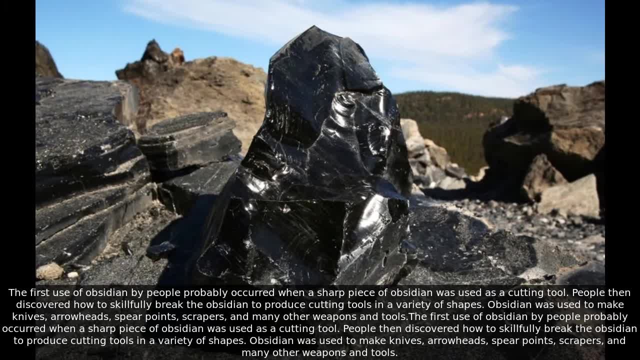 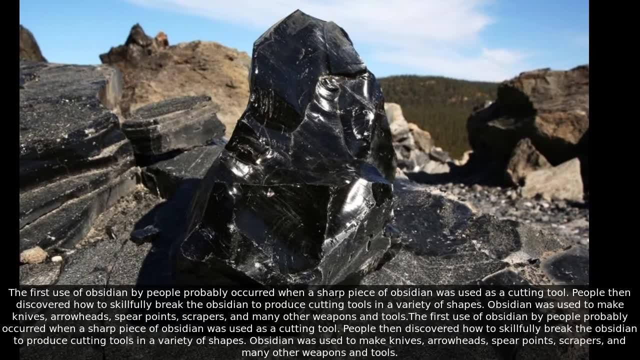 People then discovered how to skillfully break the obsidian to pieces. People then discovered how to skillfully break the obsidian to pieces. obsidian to produce cutting tools in a variety of shapes. Obsidian was used to make knives, arrowheads, spear points, scrapers and many other weapons and tools.